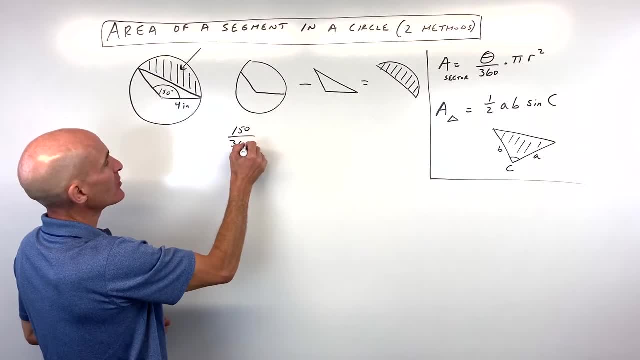 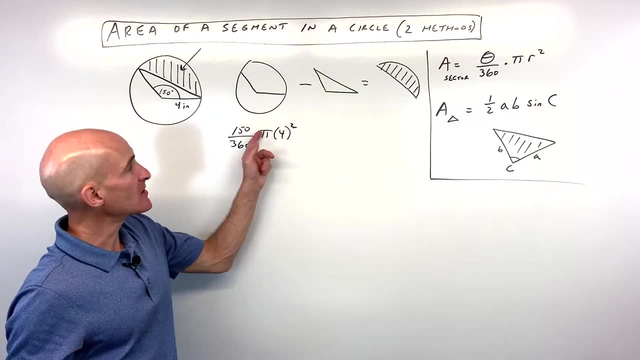 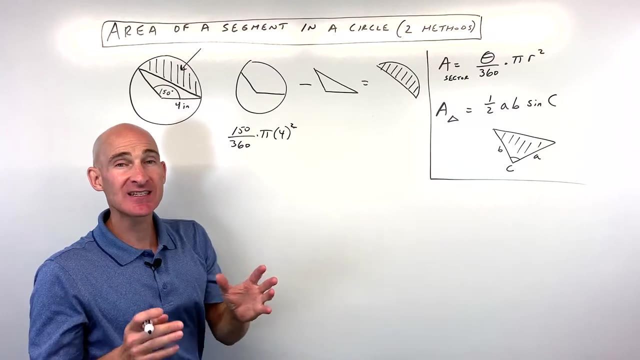 say, 150 divided by 360 times PI R squared. in this case, the radius is 4. now if you notice the PI R squared, that's the area of the whole circle. theta divided by 360, or in this case 150 divided by 360, is the fraction of the. 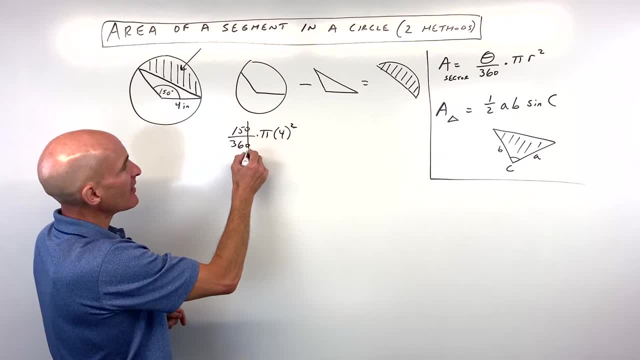 whole circle. so, for example, if we were to reduce this down by dividing by 10, and if we divide by 3 top and bottom, that gives us 5 twelfths. so this really represents 5 twelfths of the area of the circle. so we're going to divide by. 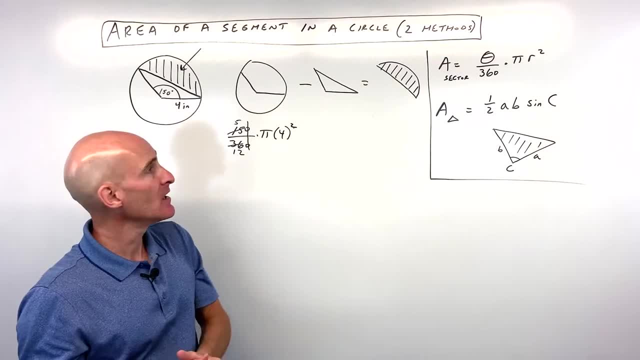 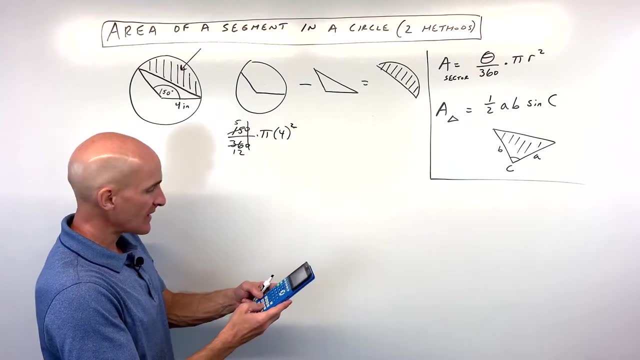 the area of the whole circle, 16 PI. so let's go ahead and simplify that down a little bit further and I'm just going to use 3.14 for PI or I'm just going to use the PI key. so we're going to say 5 times PI, times 4 squared, which is 16 divided. 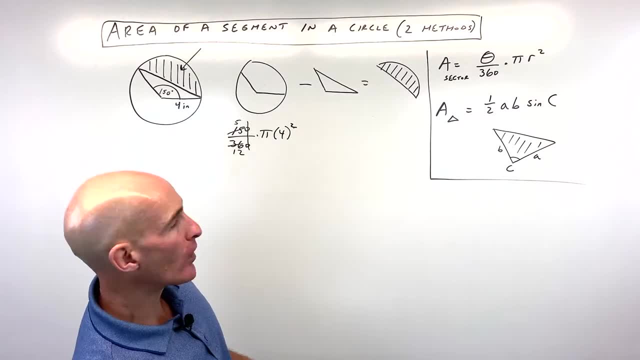 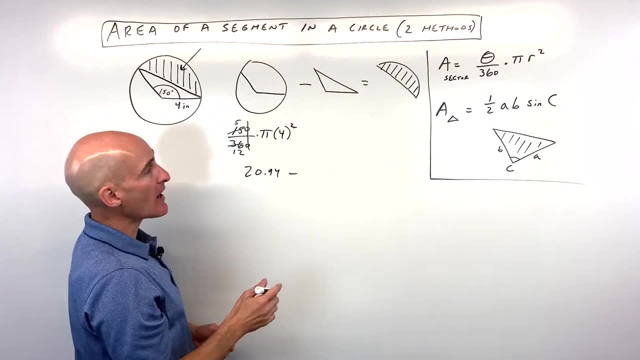 by 12 is going to come out to 20.94. I'm just rounding a little bit here. so 20.94 is the area of our sector minus now the area of our triangle. we're going to use this formula here: one half of the area of our sector minus now the area of our. 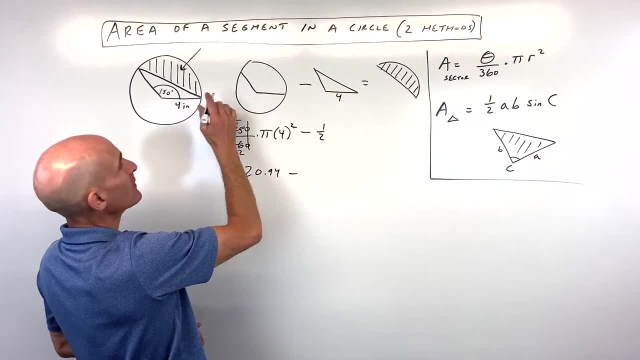 triangle. we're going to use this formula here: one half of the area of our triangle. we're going to use this formula here: one half. now, a, you see, is 4, be here is also 4, since the radius is always 4, so we have one half 4 times 4 times the. 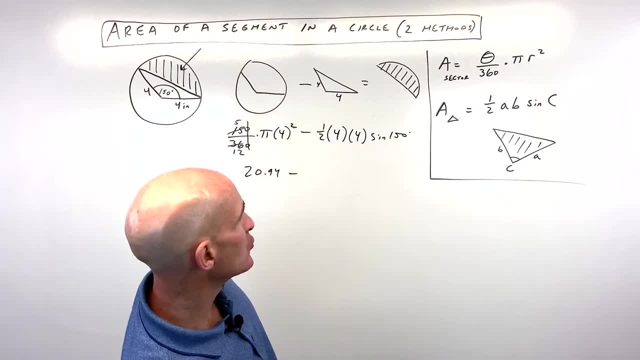 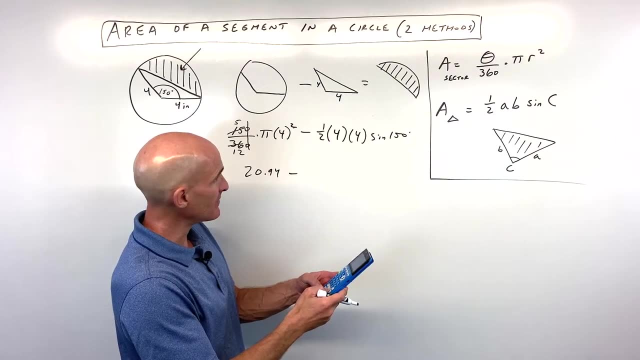 sine of the included angle, which is 150 degrees. when you're doing this, make sure you're in the degree mode on your calculator. so let's see one half times 4. times 4, which is 16 times the sine of 150, comes out to 4, so you can see 20.94. 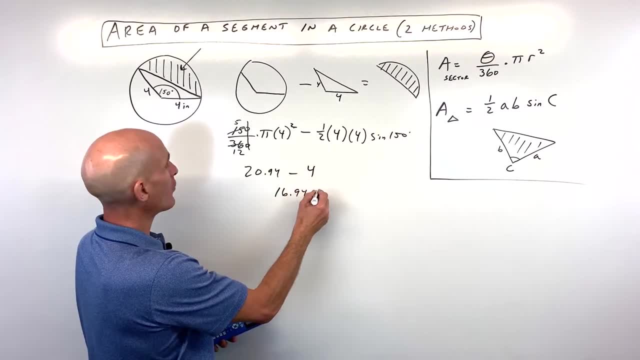 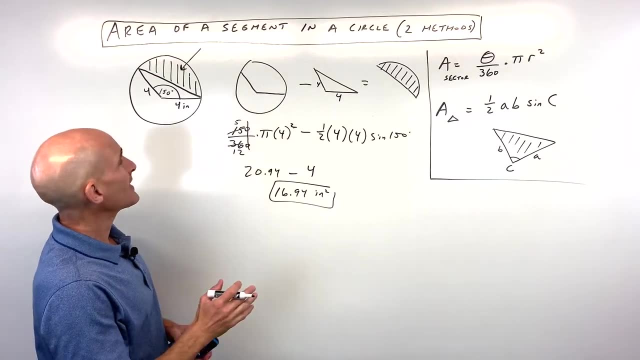 minus 4 is 16.94, 94 inches squared, That's the area of the segment. Now you're saying, Mario, what about what's the second method? Well, the second method is what you can do to find the area of this triangle. 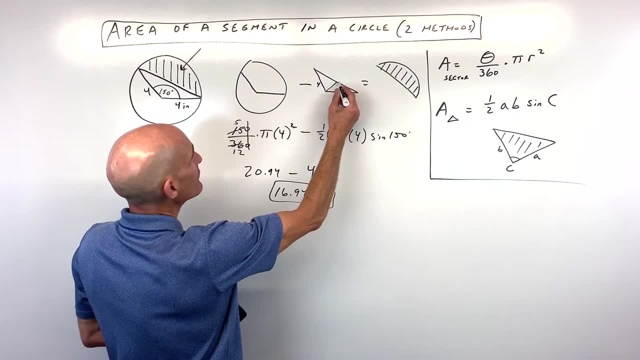 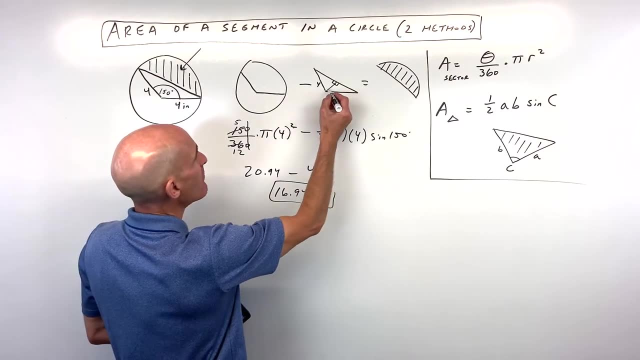 is, you can drop a perpendicular like so: Okay, Now see how this is an isosceles triangle. So what's going to happen here is this is 150 degrees. We're actually bisecting that angle, So it's going to be 75 degrees, 75 degrees, And then what you can do is you can do some. 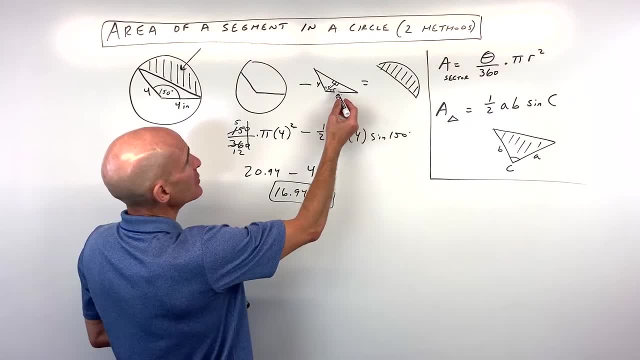 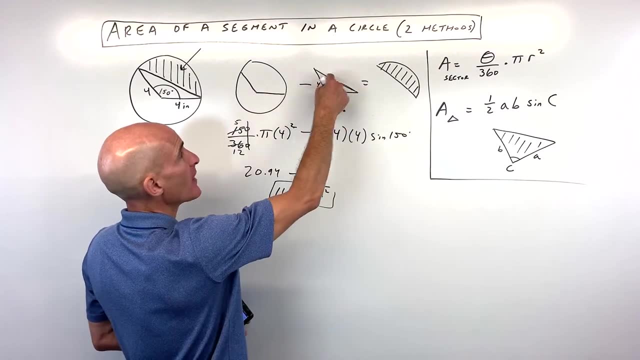 trigonometry, Okay, Sine and cosine, And you can find out what's the height of this triangle which is right here, What's this length here, And you can double it to get the base And then you can do one half base times height to find the area of that triangle. So you want to see that. 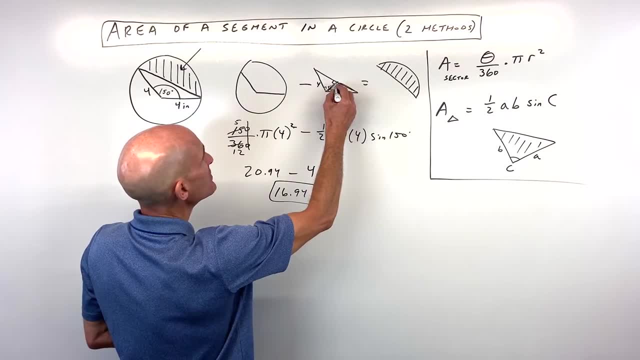 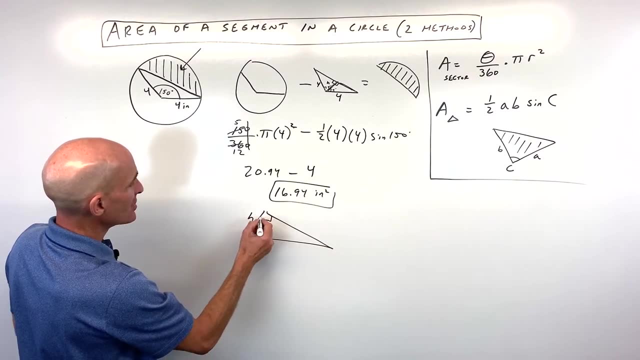 part. Okay, So I'll show you that part. So I'm just going to call this piece right here H. Okay, So let's draw that triangle a little bit bigger so we can see it. So it looks something like this: So this is going to be H and this I'm going to call this just X. So we have 75 degrees. 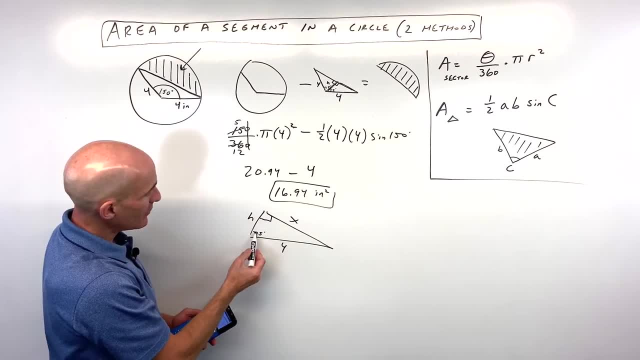 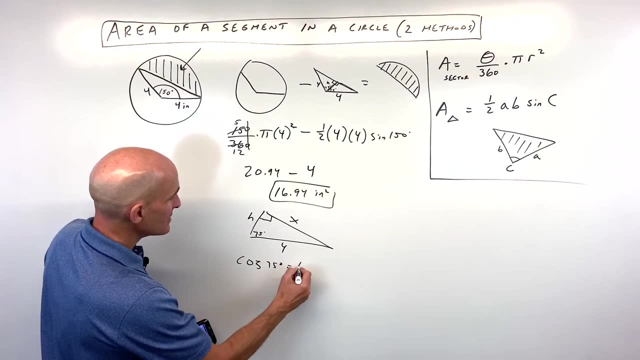 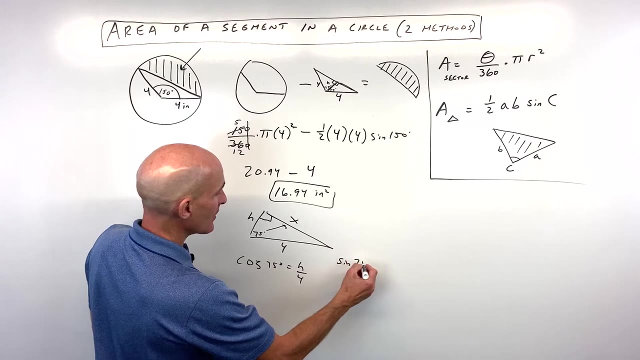 the hypotenuse here. And what trig function ties together adjacent and hypotenuse? That's cosine. So we have: the cosine of 75 degrees is equal to H over 4.. And what trig function ties together opposite and hypotenuse? That's the sine. So we have sine of 75 degrees equals X over 4.. And now, if I just 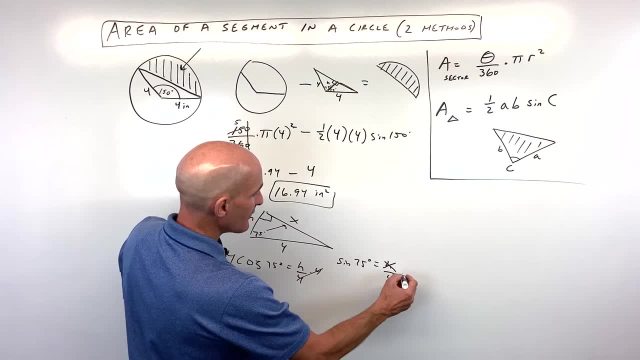 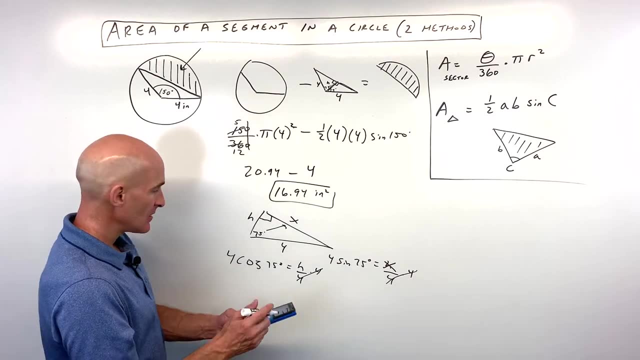 multiply both sides by 4, that gives us H. If I multiply here both sides by 4, that gives us X. So let me go Go ahead and do that on the calculator. We've got 4 cosine 75, which is about 1.035.. Okay, don't. 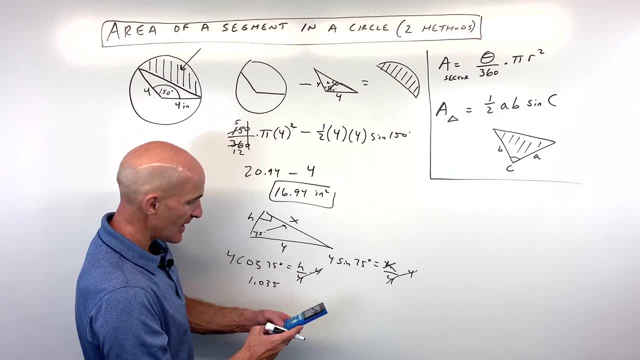 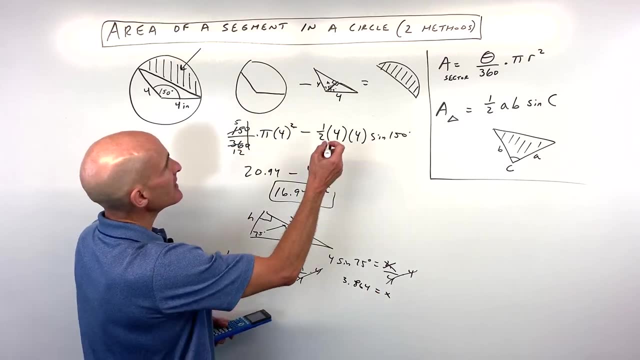 run around too much too early And we've got 4 times the sine of 75, which is 3.864.. And that's X. Now the thing is, see how we got 3.864 here. This piece here is also 3.864.. So we have to add. 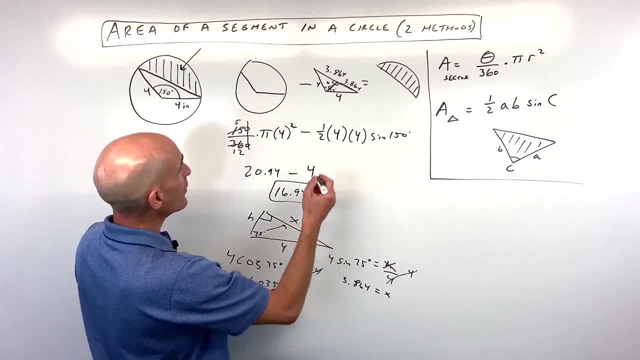 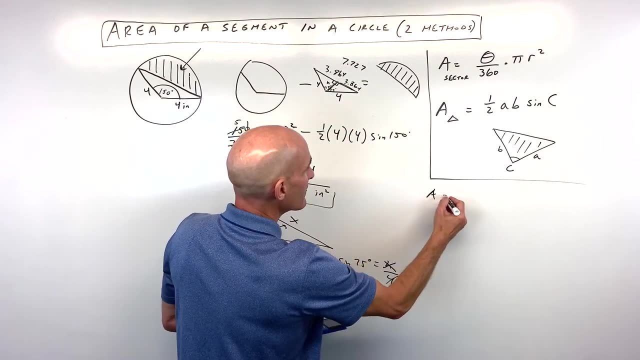 those together or multiply by 2.. So that comes out to about 7.. 7.727.. Okay, so now the area of our triangle. we know the old way of finding the area of a triangle: 1.5 base times height. we've grown up with that. The base here is going to be 7.727.. 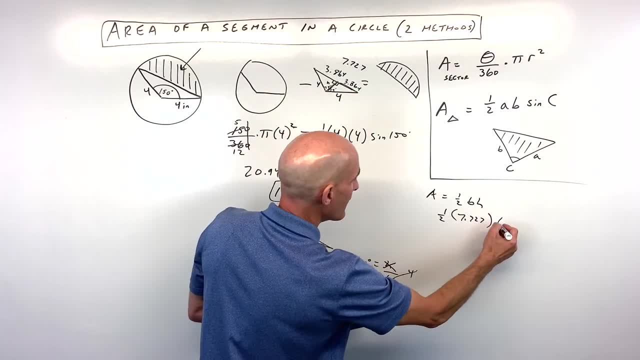 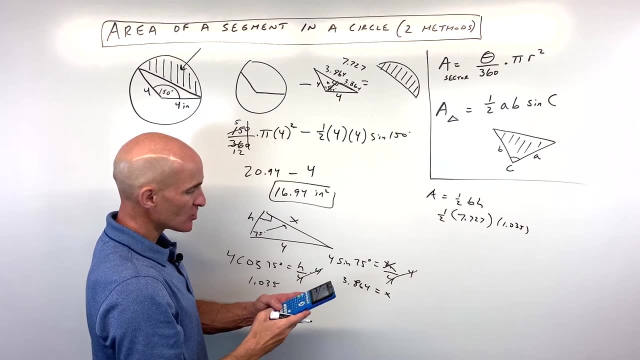 The height we said was going to be 1.035.. And if we multiply all that together, just make sure we're coming out to 4.. Okay, I'm rounding a little bit here And you can see that's the same area we got when we used the 1.5 ABC.